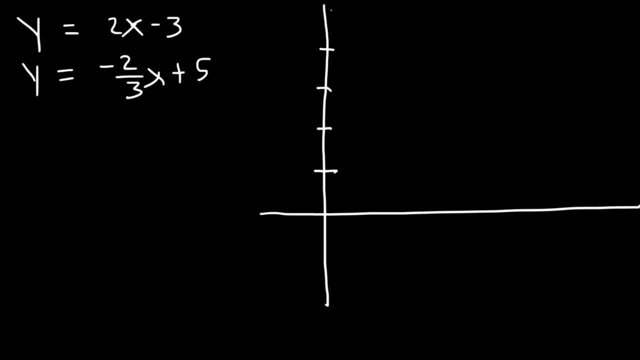 Let's go up to 5 on the y-axis And let's do the same for the x-axis. The advantage of drawing a big graph is you can clearly see where the solution is going to be. If you draw a graph with the marks closely spaced to each other, it might be difficult to see the answer. So the bigger the graph, the better it's going to be. 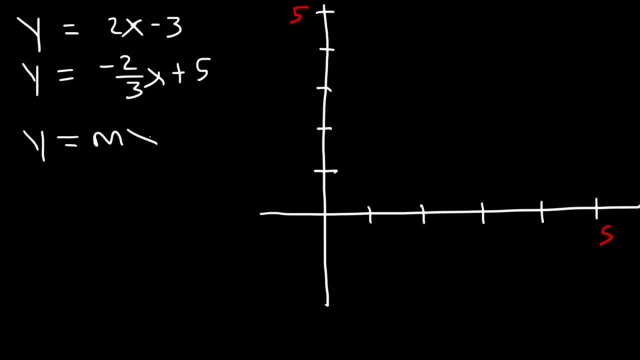 Now, if you draw a graph with the marks closely spaced to each other, it might be difficult to see the answer. So the bigger the graph, the better it's going to be. Now, each of these equations is in slope-intercept form. So, starting with the first equation, we can see that m the slope is 2, and the y-intercept is negative 3.. So we need to go down at least 3 units. 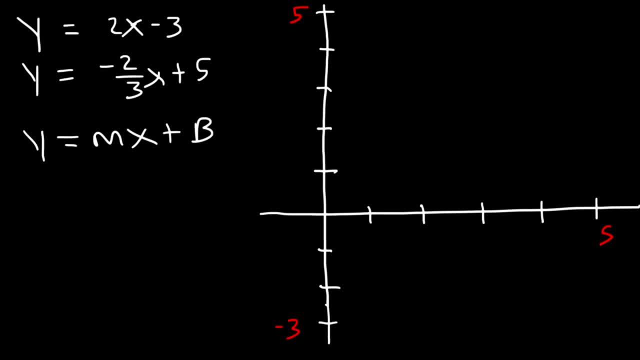 So for the first equation, the y-intercept is negative 3.. That's going to be the first point. To find the next point, use the slope. The slope is 2.. Slope is rise over run. so you have to go up 2 units and travel 1 unit to the right. 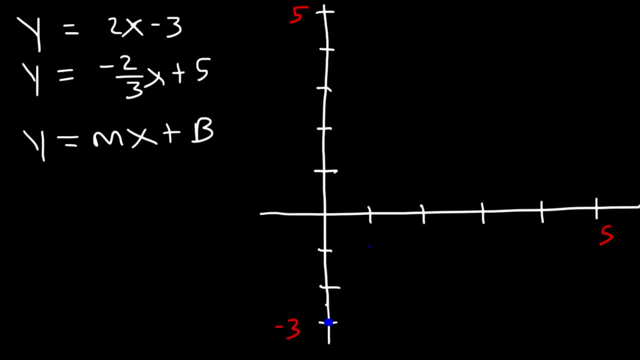 That will take us to the next point, which is 1, negative 1.. Now let's do it again. Let's go up 2 over 1.. So that's going to take us to the point 2, 1.. And then, if we go up 2 over 1, we're going to be at 3, 3.. Up 2 over 1, then 4, 5.. And that's enough for this graph. 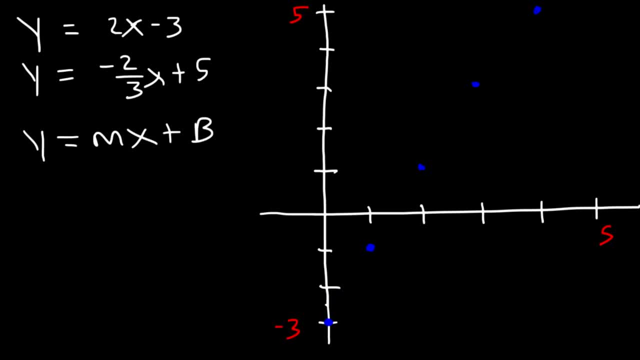 And my lines are not perfectly straight, but Let's do that again. You get the picture. Now let's graph the second equation. The y-intercept is 5.. So we're going to start at a y-value of 5.. The slope is negative, 2 over 3.. 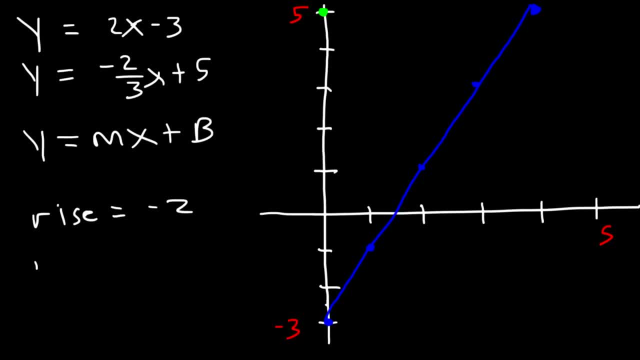 So the rise is negative, 2.. The run is positive, 3.. So, starting from the first point, we need to travel- That's the run- And then we need to go down 2 units. So that will take us to the point 3, 3, which we can see is the point of intersection. 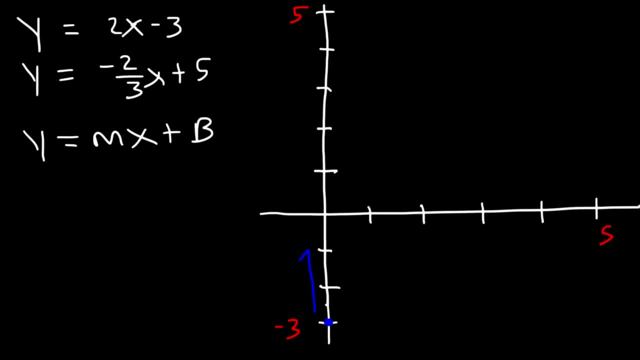 The slope is 2.. Slope is rise over run. so you have to go up 2 units and travel 1 unit to the right. That will take us to the next point, which is 1, negative 1.. Now let's do it again. let's go up 2, over 1.. 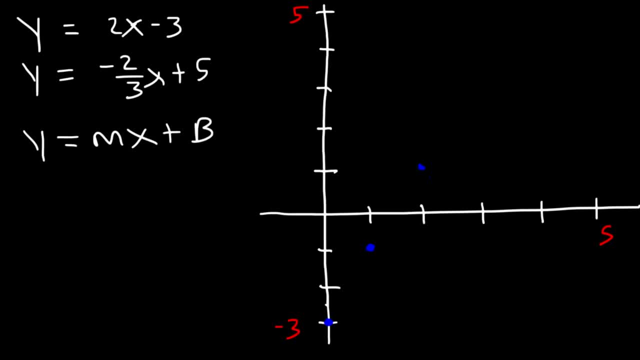 So that's going to take us to the point 2, 1.. And then, if we go up 2, over 1, we're going to be at 3, 3.. Up 2, over 1, then 4, 5.. 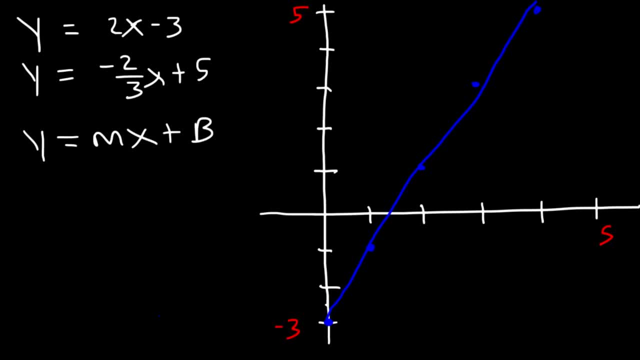 And that's enough for this graph, And my lines are not perfectly straight, but let's do that again. You get the picture. Now let's graph the second equation. The y-intercept is 5.. So we're going to start at a y-value of 5.. 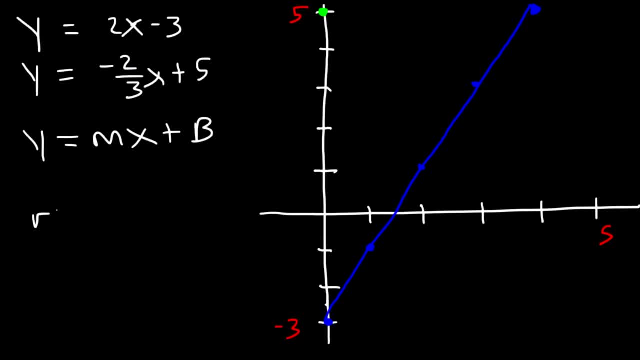 The slope is negative 2 over 3.. So the rise is negative 2, the run is positive 3.. So, starting from the first point, we need to travel 3 units to the right. That's the run- And then we need to go down 2 units. 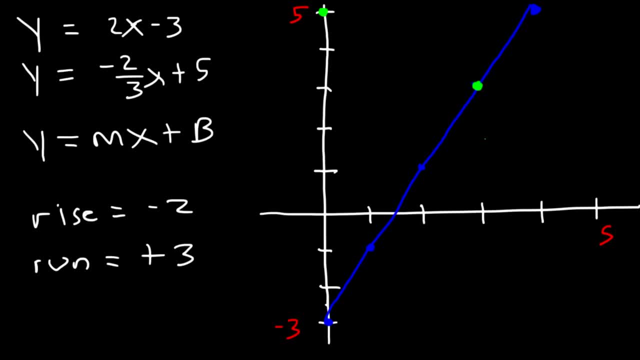 So that will take us to the point 3, 3.. Which we can see. it's the point of intersection, But let's continue graphing it. Now we need to go 3 to the right down 2, but we're out of space for that. 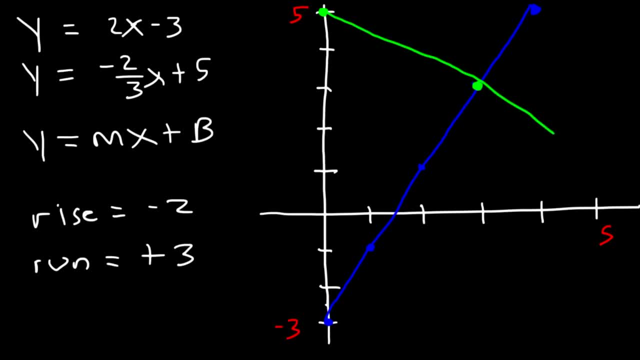 So let's just use these two points, And so that's going to be the graph, And then we're going to go down 2 units. That's the run, The total line of the second line. So the point of intersection is 3,3.. 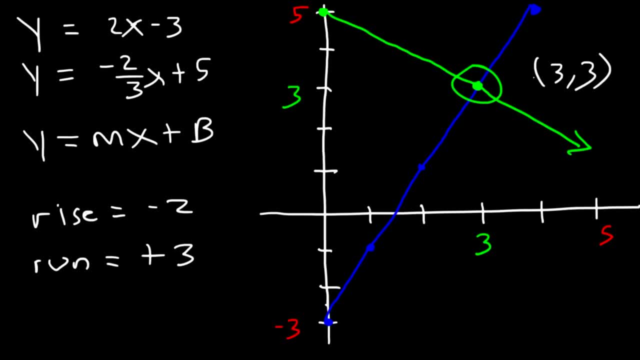 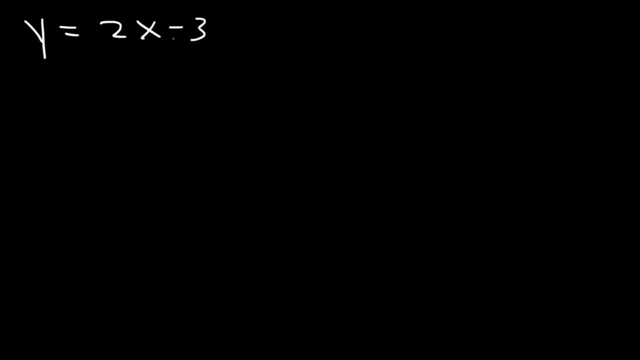 So, therefore, that's the solution to the equation. Now let's check it. Now let's solve this by substitution. Let's replace y 2. with 2x minus 3. So, therefore, 2x minus 3 is equal to negative 2 over 3x plus 5..